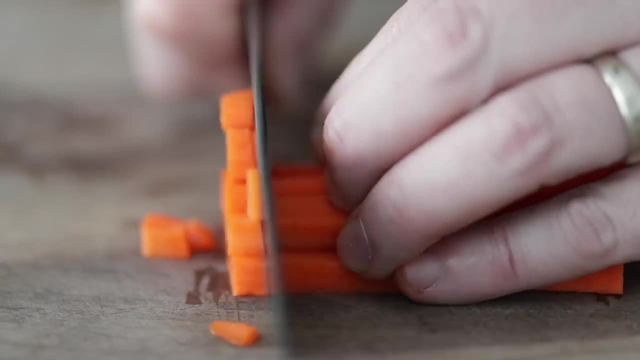 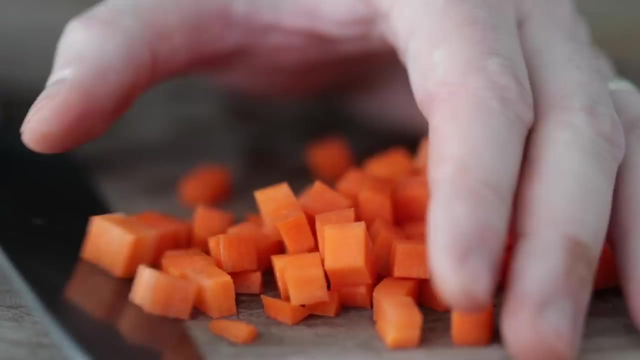 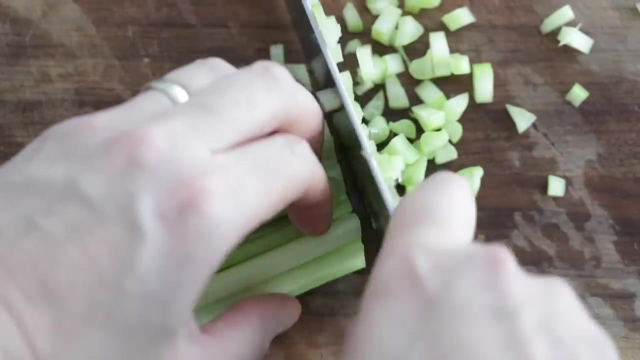 That we want to peel up And, just like the onions, we want to small to medium size dice these. Next, I have two ribs of celery that we are also going to small to medium size dice And, real quick, why have I always called these stalks of celery? A stalk is a bunch. What I've 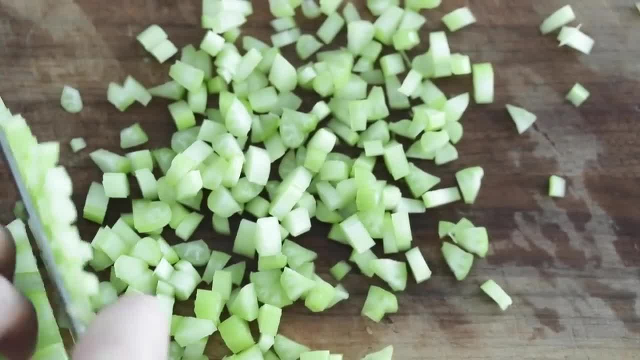 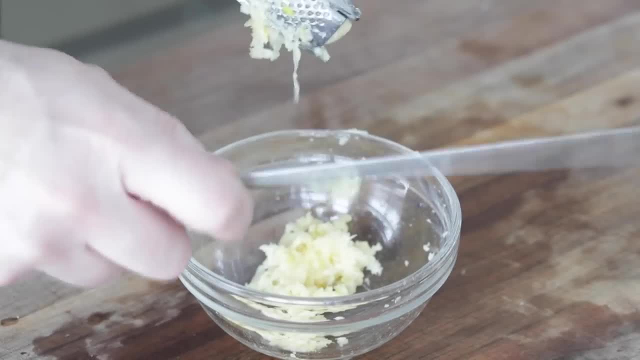 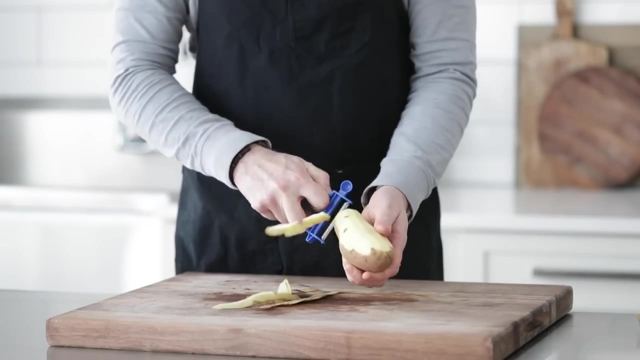 always meant is a rib, So two ribs of celery small to medium size dice For garlic. you already know I'm going to run three cloves right through this garlic. Next I have one large baking potato You could substitute out for two small russet potatoes. 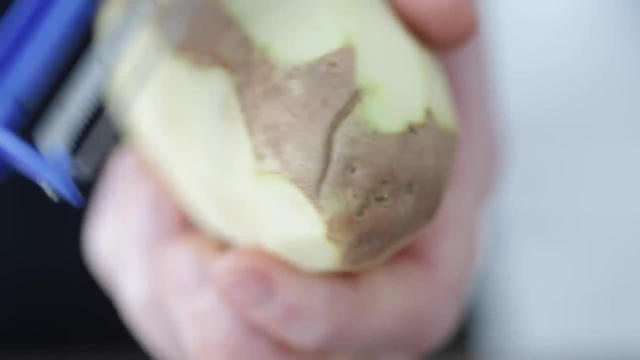 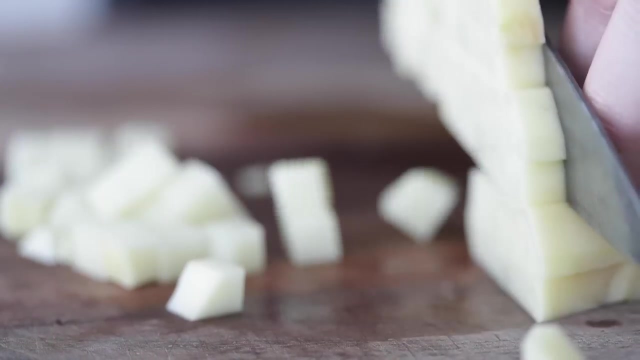 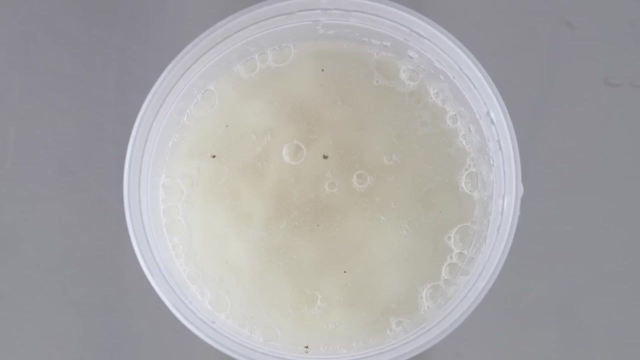 or three red, new or golden Yukon potatoes, Peel those up and then again medium size dice these To take care that these do not brown. we're just going to add them to a container with cold water or when it comes time to kneading them. 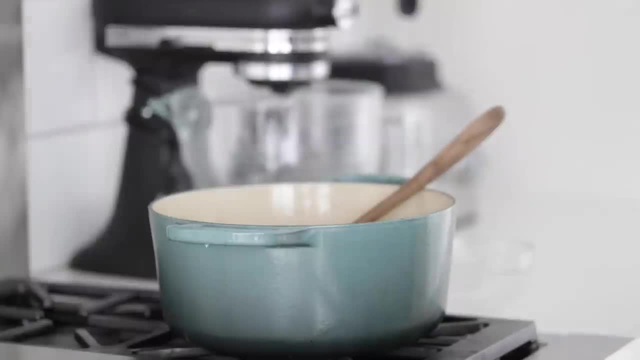 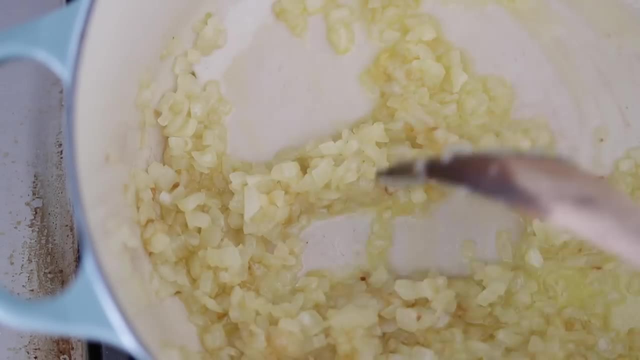 we'll just drain them off, Set them to the side. Let's go back over to the pot. Let's just have a look at our onions. It's been about 15 minutes or so. Let's give it a quick stir, Starting to become translucent- not quite brown yet. 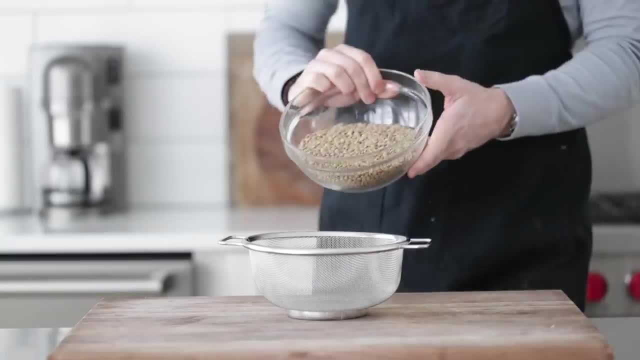 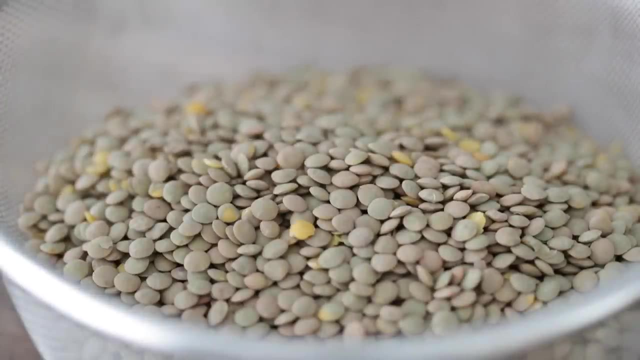 The flavor is still in the work- Great timing. We have three cups of green lentils. You can also use red, yellow or brown lentils, Although red and green seem to be most common at the local grocery store. the one that I would not recommend are French lentils. 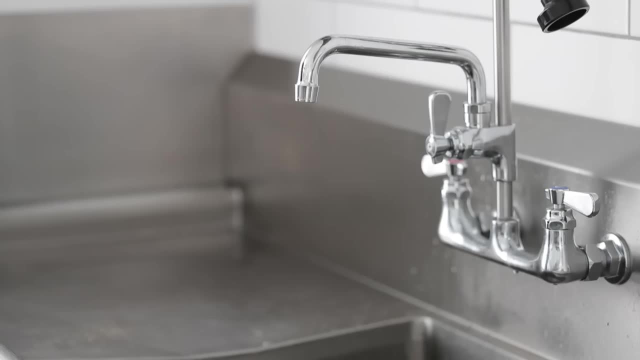 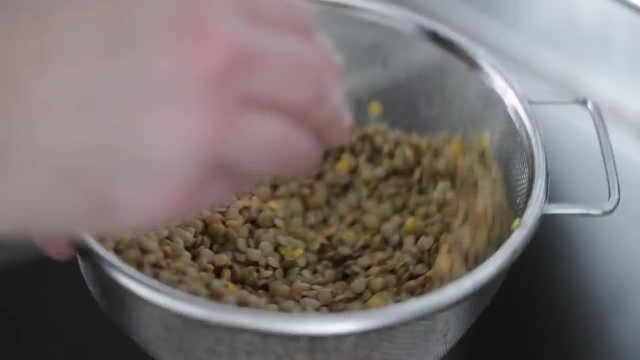 because they don't break down and be really hard to get the right consistency in our soup. Let's head over to our sink. What we wanna do is rinse these under cold water, maybe just for a minute. Sometimes lentils can be really dirty. 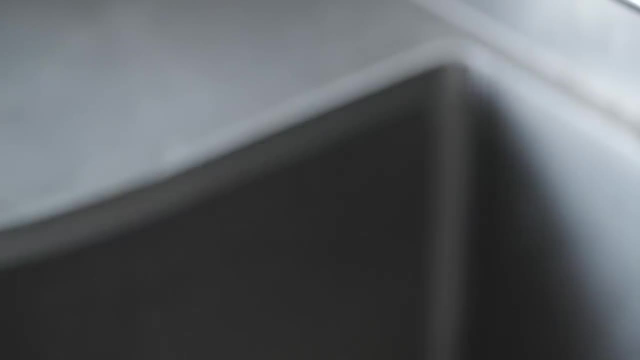 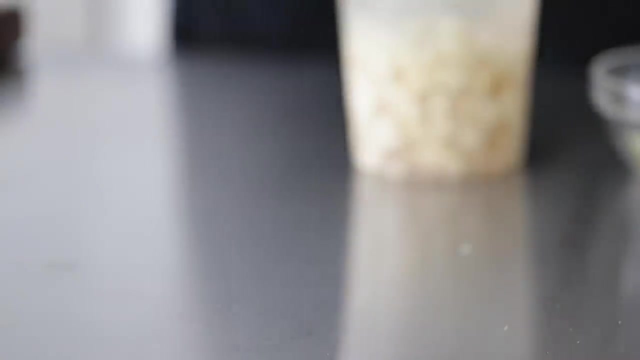 so give them a quick rinse, a good shake. We are gonna set them to the side in a bowl until we need them. Now let's go back over to our prep area. We've got our carrots, celery potatoes and garlic. 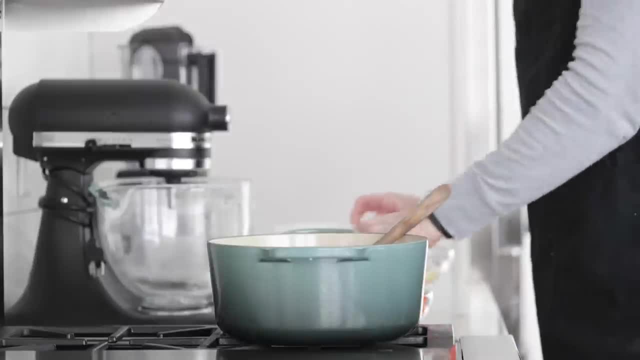 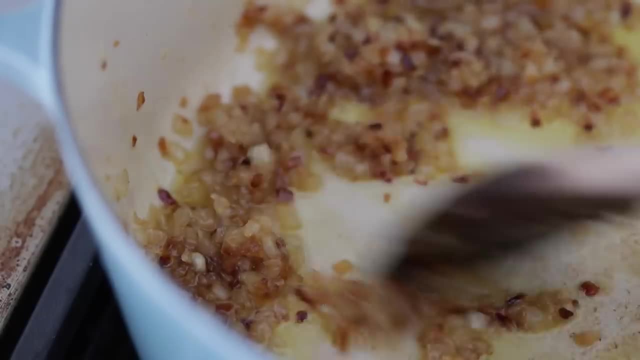 We're gonna take all these goodies back over to our cooktop. Let's have another look at our onions. Give them a quick stir. see how they're doing Absolutely perfect Browned tender. so much goodness in these. Again, I can't say enough. do not skip this part. 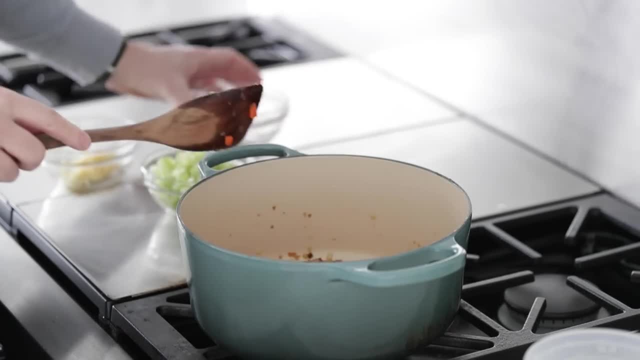 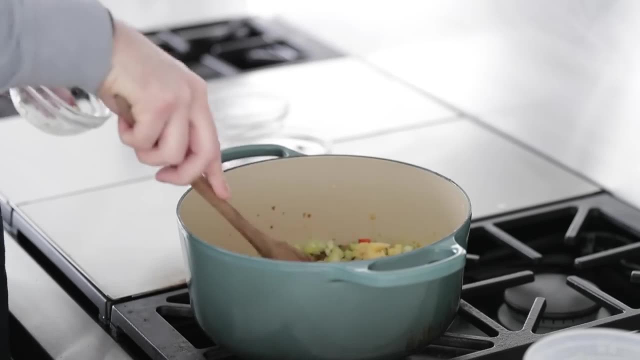 Now what we're gonna do is add in our carrots, followed up by adding in our celery, and then, of course, last but not least, let's add in our finely minced garlic. We're gonna turn the heat up to medium here. These vegetables are a little bit bigger. 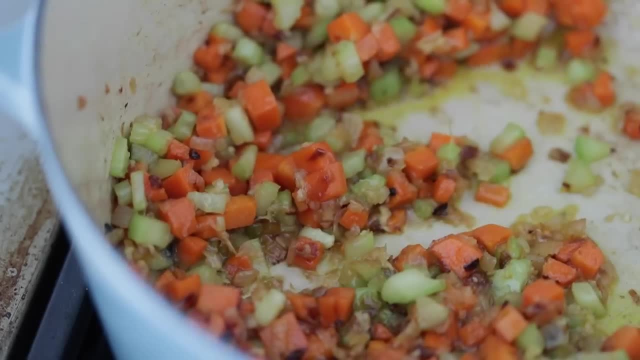 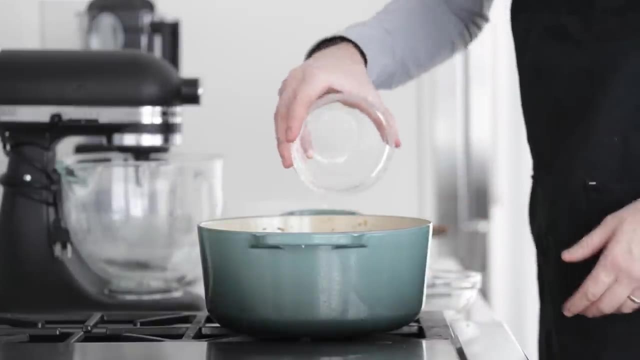 You wanna get a nice light brown on them, just like this? Perfect. Now for a little bit of spice. I'm going to add in one and a half teaspoons of ground cumin and one teaspoon of ground coriander. I like adding it at this stage. 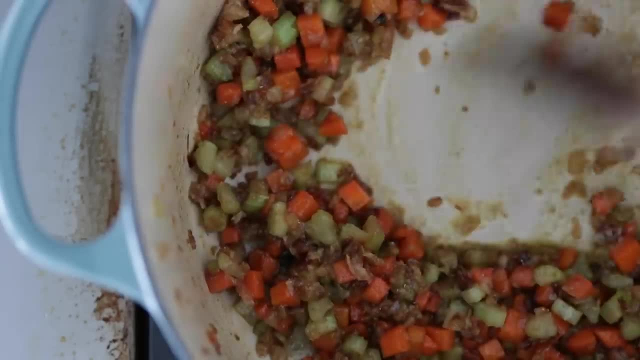 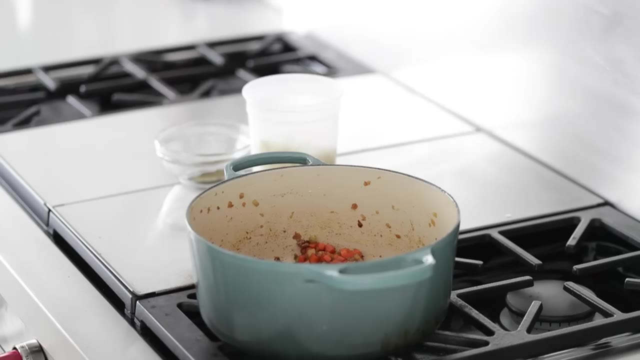 because it sort of gives a little toast while we're sauteing in the vegetables. Also at this stage, if you want, you could deglaze with about a half cup of white wine, Chardonnay or Sauvignon Blanc. 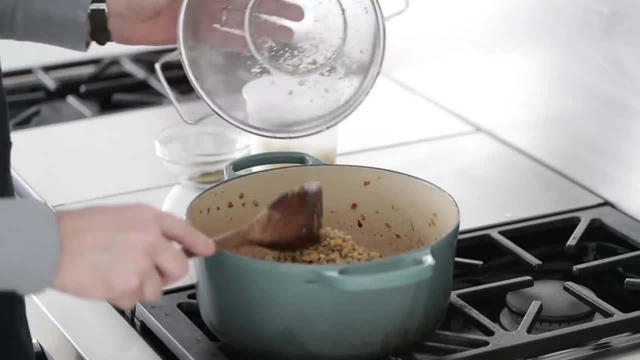 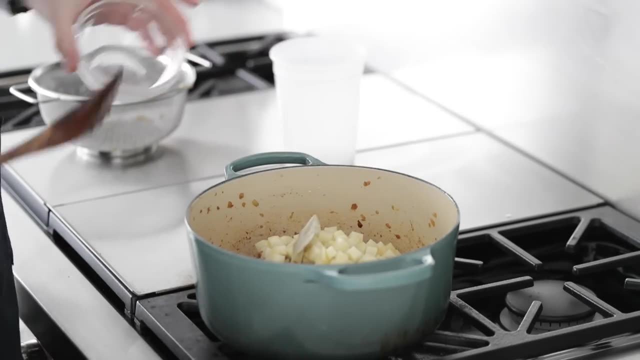 Now let's grab our lentils, Let's pour those in there, followed up with our potatoes. Yes, I already drained the water off. We are next going to add two bay leaves. You could also add a can of drained chickpeas right now. 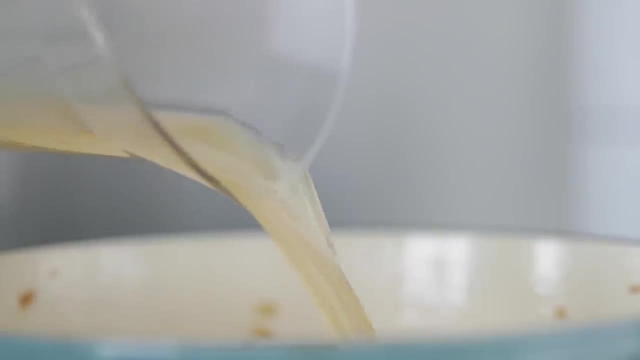 if you'd like. Next, I have nine cups of chicken stock, but if you wanna keep this vegetarian vegan, feel free to use water or simply vegetable stock. Let's give it a quick stir just to mix all of those ingredients together, get them infusing. 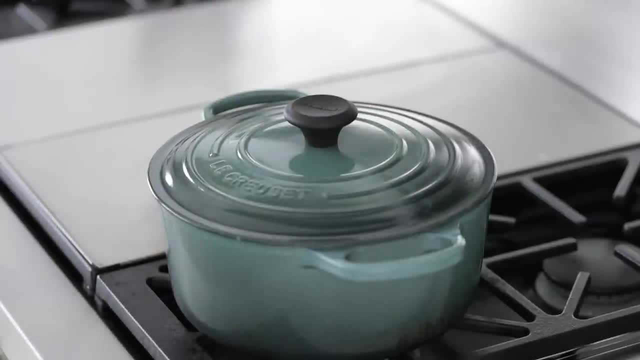 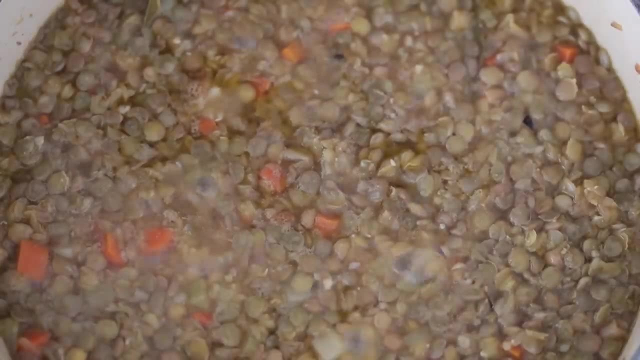 We're gonna add a lid, turn the heat to low to medium. It's gonna take about 45 minutes for these lentils to cook through and to become nice and tender. At that time we'll come back and take a peek. Yep, absolutely. 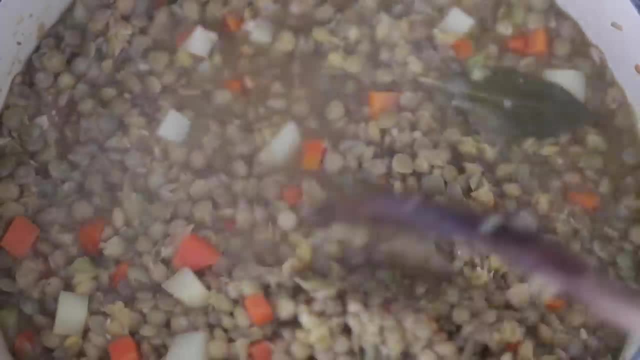 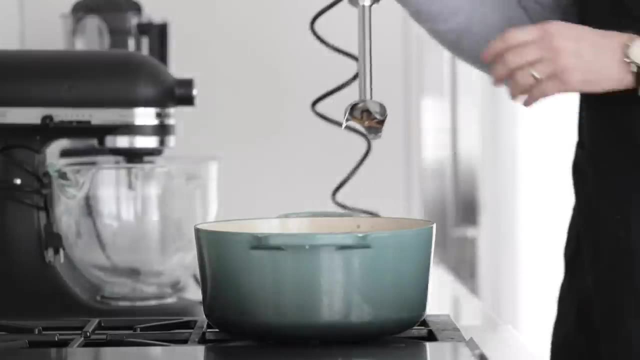 Perfect. Let's just give it a quick stir and move some things around. Looks excellent. Now, don't forget, we want to remove the bay leaves out of there. You can discard them. No need to keep them. Now I have an immersion blender. 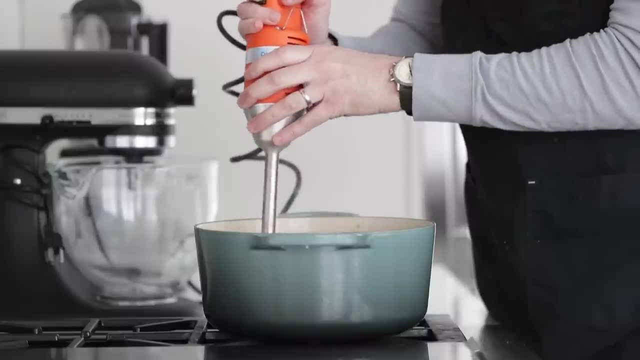 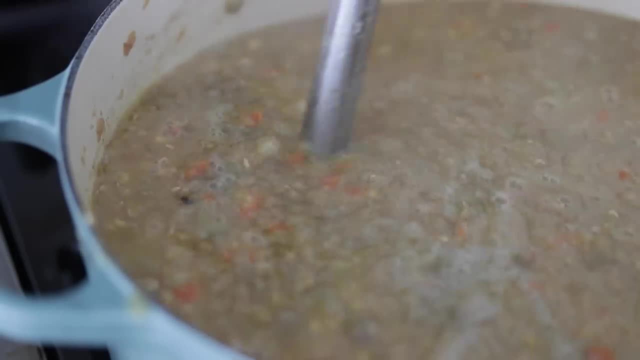 which we're gonna add in there and give a series of pulses. Now, we don't wanna completely break down this soup, so it's completely smooth. We want it to have some texture, So the series of pulses is what you should do. Also, if you don't have this, take half the soup. 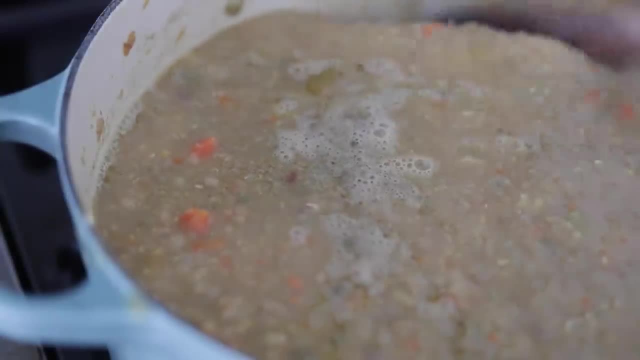 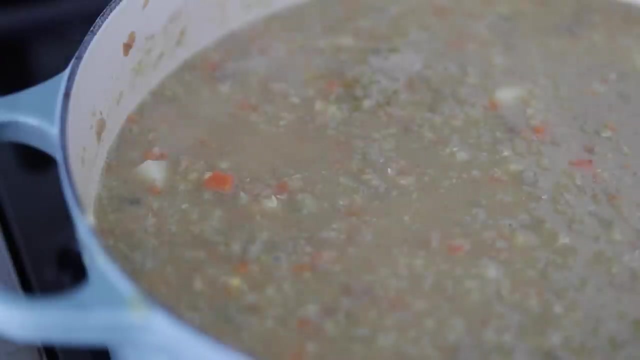 run it through a blender, get it nice and smooth, add it back in there. That'll be the perfect consistency, just like this. Also, in addition, if you wanted to, you could add two cups of packed baby spinach at this stage for a little green.